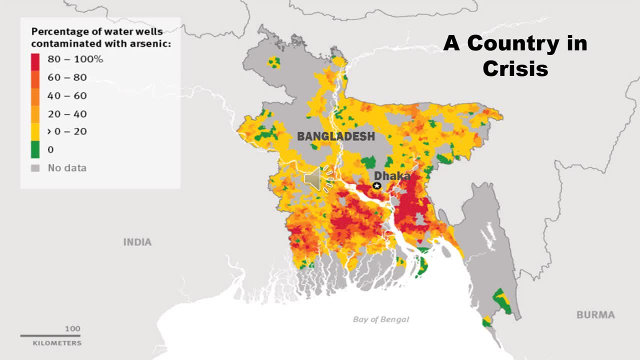 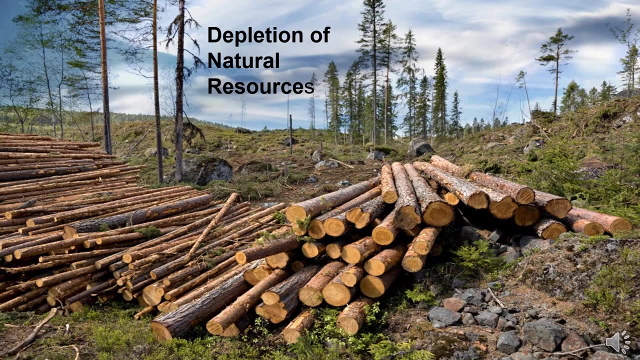 43,000 people die each year from arsenic poisoning and this problem has been known for 20 years. The government has been heavily criticized in the response in prevention and treatment. Veryò. Population increases have led to resource diminishment and an increase in competitive stress on basic resources. 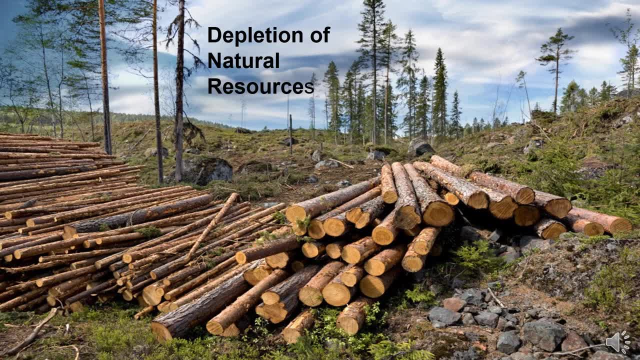 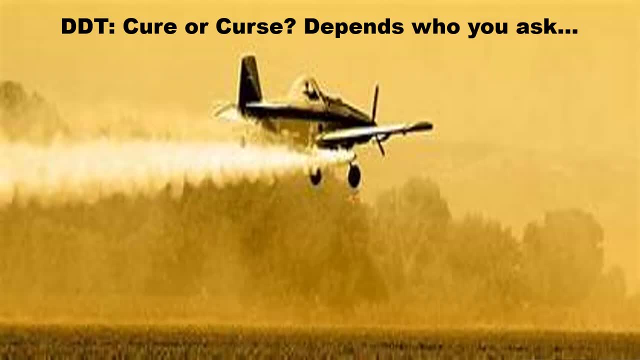 In a study by the UNEP Global Environmental Outlook, every person requires a third more land than the plant can supply. DDT is an extremely controversial pesticide that was used mainly to combat malarial mosquitoes during and after World War II. While it effectively killed pests, it bio-magnified in the food chain, ending up in humans. it reduced malaria, while at the same time it wreaked havoc on other parts of the environment as well. 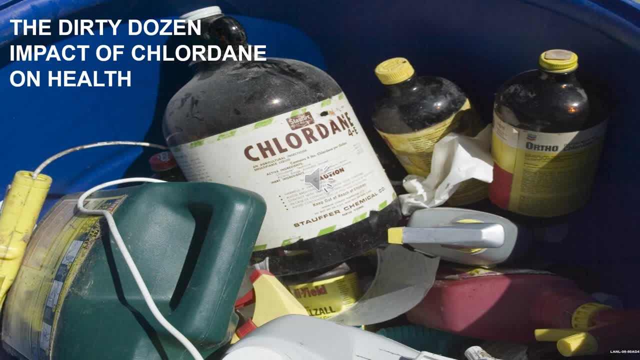 Everyone in the United States has been exposed to Chlordane, a man-made pesticide that was used from the late 40s to late 80s. It was mostly used in the soil around homes to kill termites in the 80s, but was also used on farmland in the 1960s, where it would remain in the soil for 20 years. 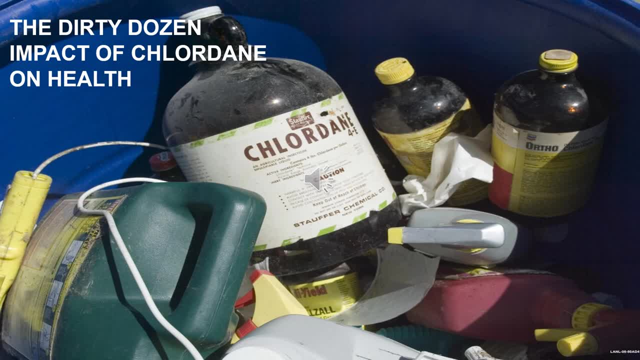 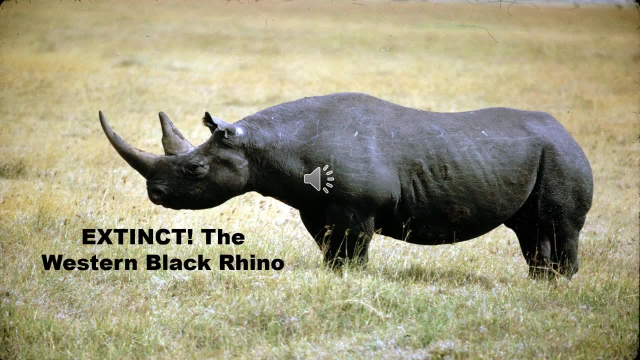 It was phased out in 1988 after it was found to build up in body fats and cause cancer. Western Black Rhinos once roamed central and western Africa in the African savannas. During the first half of the 20th century, sports hunting, industrial agriculture and traditional Chinese medicine dwindled their numbers. 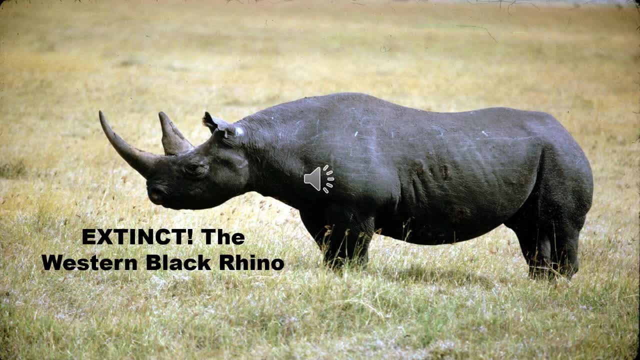 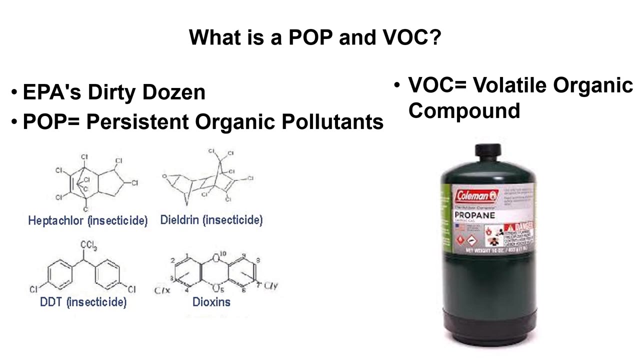 Through strict laws. in the latter half of the 20th century, their numbers rebounded. Unfortunately, illegal poaching for the rhino's ivory tusks devastated the Western Black Rhinos to the point of extinction In 2011. Pop are the chemicals used in pesticides that remain in the environment for long periods of time. 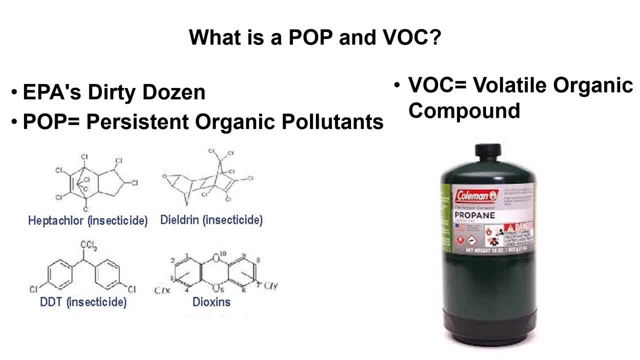 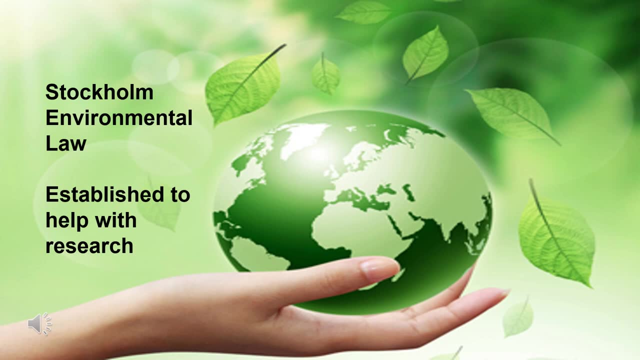 and accumulate in fatty tissues of living organisms and have a harmful impact on human health. Vocs are used in gas cleaning and painting. They can be harmful to the health of humans and create photochemical smog. The purpose of the Stockholm Environmental Law is to contribute to a sustainable 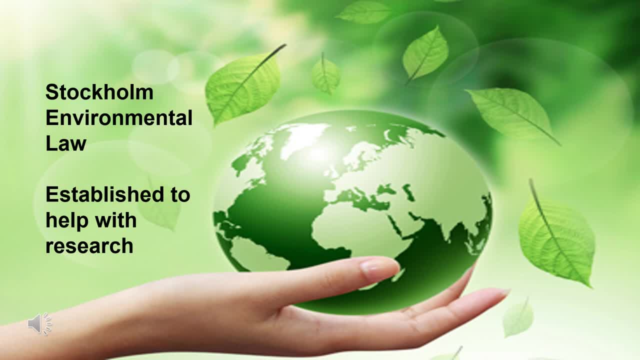 sessions for prevention of better environmental control and to improve health and liberals products. joangan of Sockholm. environmental law is to contribute to a sustainable development at the national and international level for the protection of human health as well as the environment. This law covers research as: 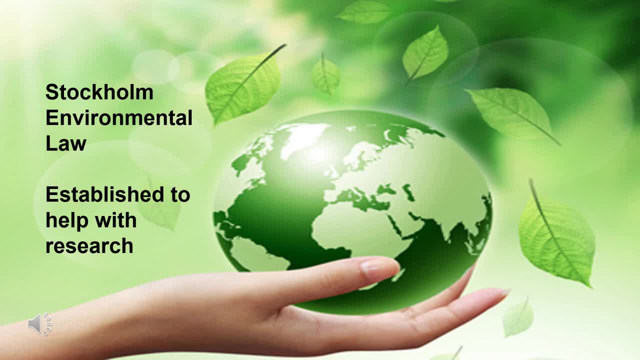 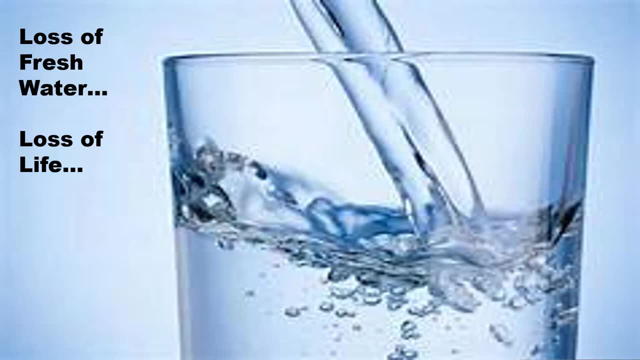 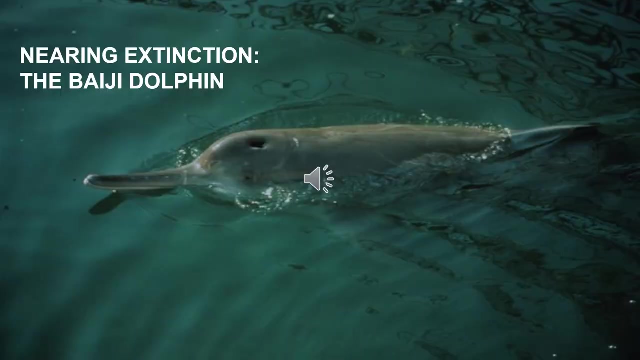 well as education. Without fresh water, there's no life. Through overuse of water for unnecessary uses and the pollution of perfectly good water, we humans have successfully depleted a large portion of world's fresh water. Greed is the fuel that feeds this fire. The Baiji River dolphin has lived for 20 million years Within a few. 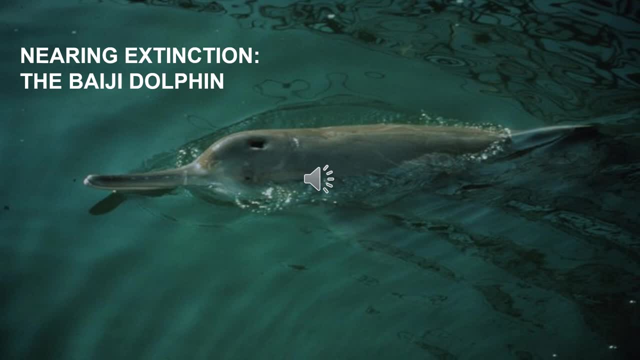 decades it has gone from a secure population to extinct- the first extinction of a large mammal species in 50 years, and it could have been avoided. It was led by the industrialization of China in the 1950s and an unsustainable 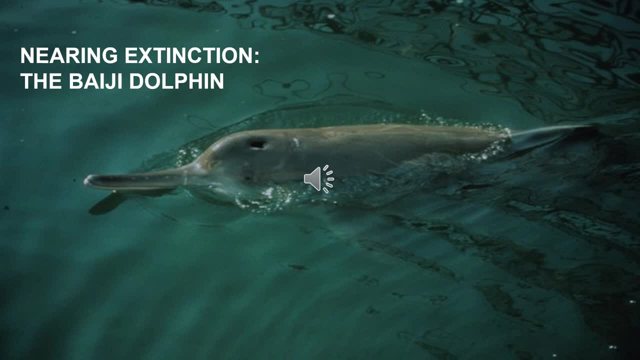 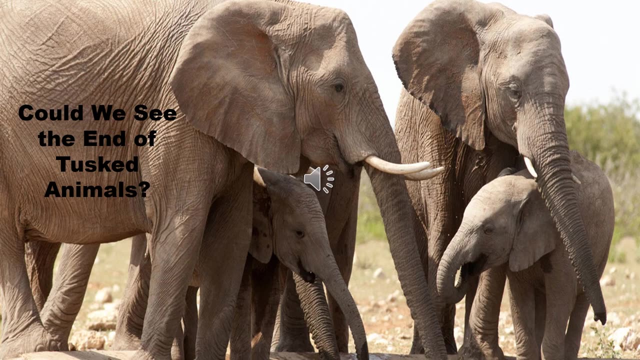 bycatch of fisheries. alongside habitat degradation, Poaching is illegal all throughout Africa. that has been on the rise since 2007.. Due to the lucrative ivory trade, elephants and rhinos are the most heavily targeted animals, leading to the extinction of several species. Luckily, 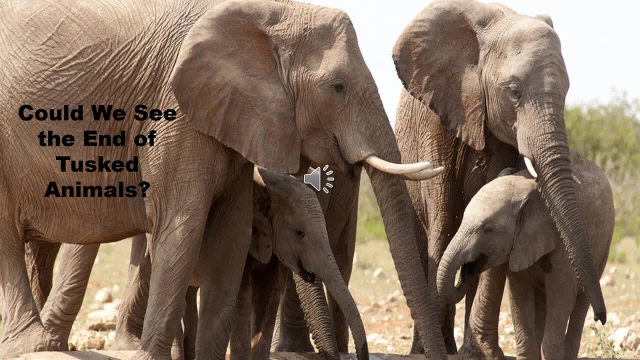 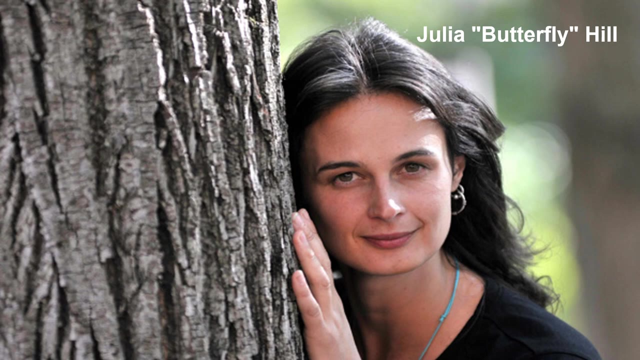 there has been a pushback against poaching, with the creation of reserves and, in some cases, continual armed guard of animals. This has led to the increase of animal population. Julia Butterfly-Hill wanted to bring attention of preventing clear-cutting of ecologically significant forests. She lived in a tree for two years. She sought to. 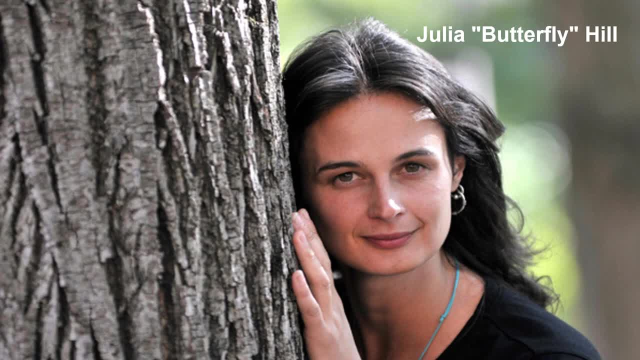 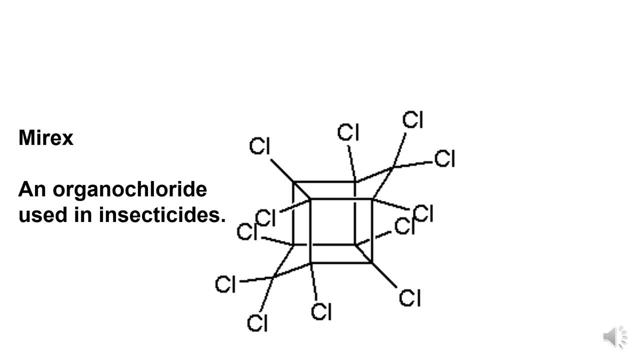 prevent the deforestation, draw media's attention to PL's disregard for the environment and educate the public about the role forests play in stabilizing hillsides. Mirex is an organochloride that was used as an insecticide specifically for controlling fire ants. It was eventually banned after it was discovered that the 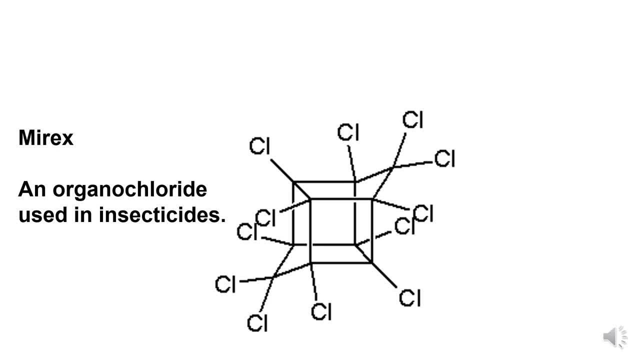 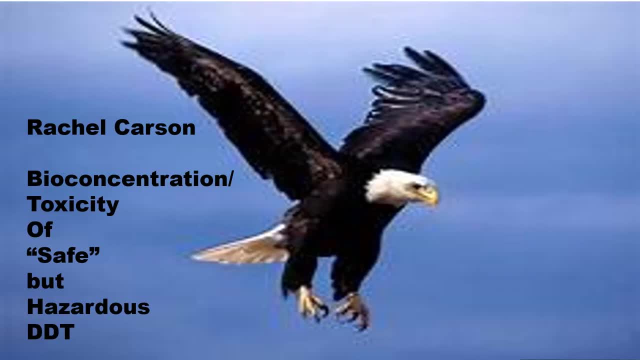 compounds would accumulate in an organism as it progressed up the food chain and would interfere with estrogen-mediated functions in the body. In 1962, Rachel Carson wrote Silent Spring, telling the story of synthetic DDT destroying populations including bald eagles. This led to a DDT outlaw. Bald eagles grow to 14 pounds with an 8-foot wingspan. In 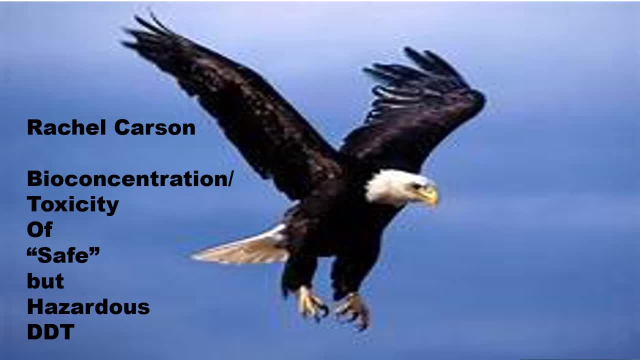 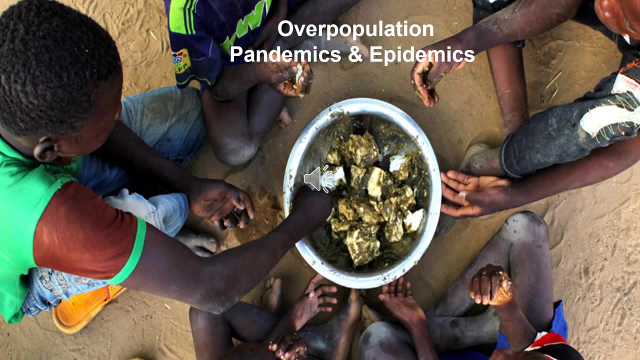 1963, 417 nesting pairs still lived in the lower forty-eight. Now, more than 9700 pairs lives in the lower forty-eight. A Changing Environment can lead to a shortage of resources, leaving an estimated 3.7 billion people malnourished. 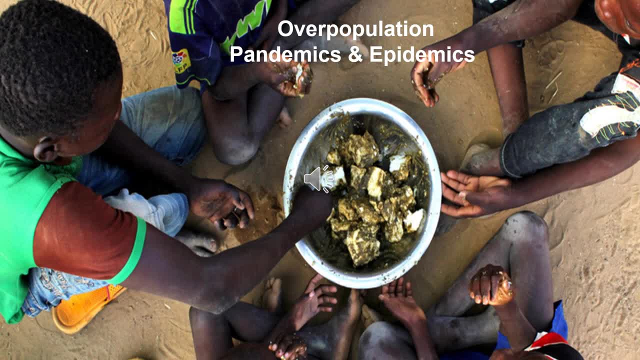 This leads to a susceptibility to disease and, combined with the reality of a planet overpopulation and lack of access to health care, the potential for an increased possibility of epidemics and pandemics is created. In countries with the fastest growing population, they also have some of the lowest life. 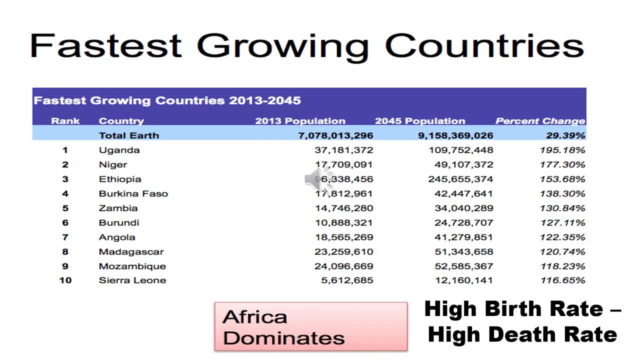 expectancies on average. This is mostly due to a lack in clean water and food, leading to malnutrition and decrease of the quality of life. This was common in England before the Industrial Revolution. Once the Industrial Revolution hit, the quality of life increased, leading to an increase. 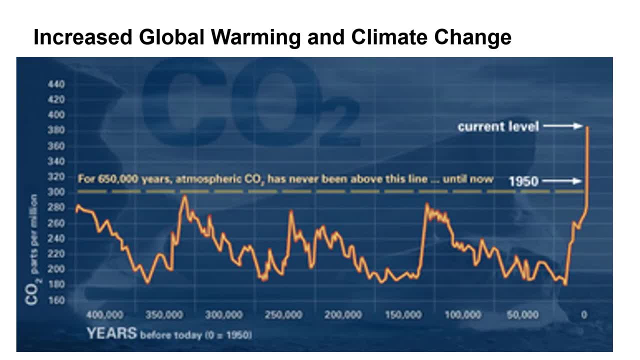 in life expectancy as well. Increased global warming and climate change is due to the buildup of human-generated greenhouse gases in the atmosphere. Climate change is a result of global warming. Human activity, most notably over the past century, has led to a rapid increase in the 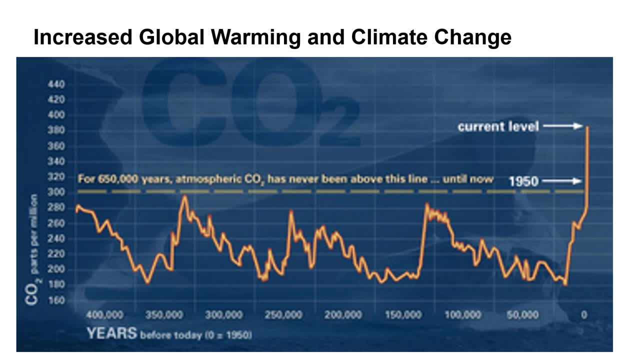 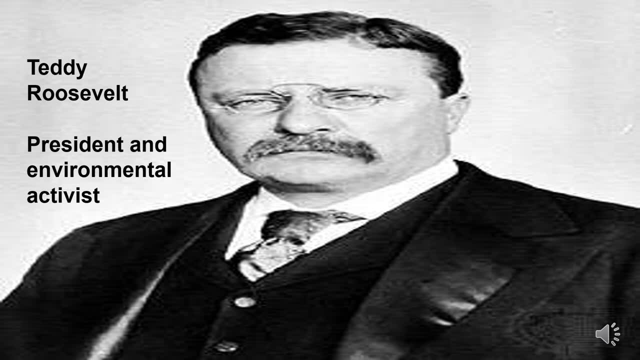 global average surface temperature due to greenhouse gases released by burning fossil fuels and cutting down trees. Roosevelt, being a sport hunter, noticed the decimation of bison in the United States, as well as the loss of elk, deer and other game. Roosevelt, to preserve the life in the wild, established 150 national forests, 51 federal 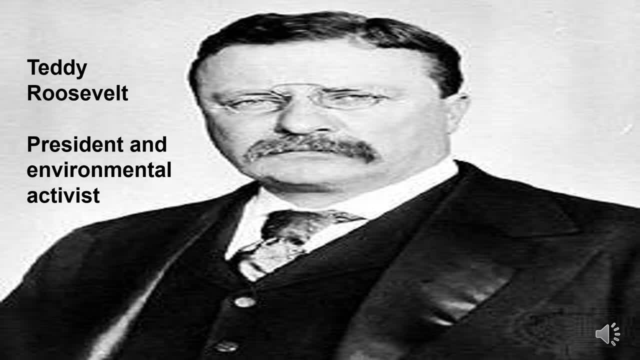 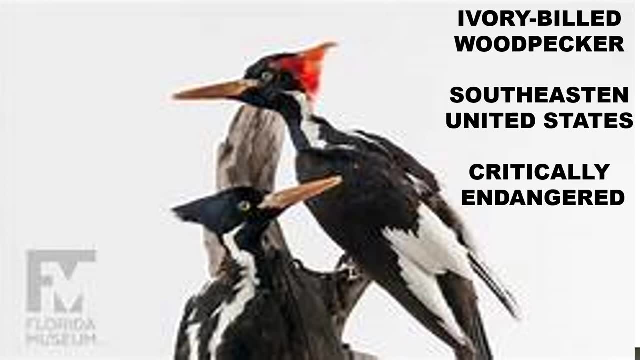 bird reserves, 4 national game preserves and 5 national parks. The ivory-billed woodpecker is one of the world's largest woodpeckers, at about 20 inches long and 30 inches in wingspan. It has a long tail. 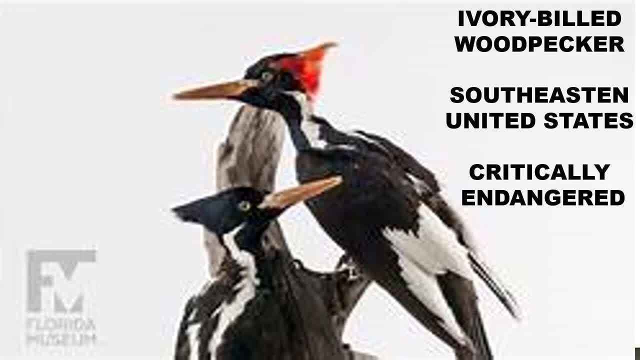 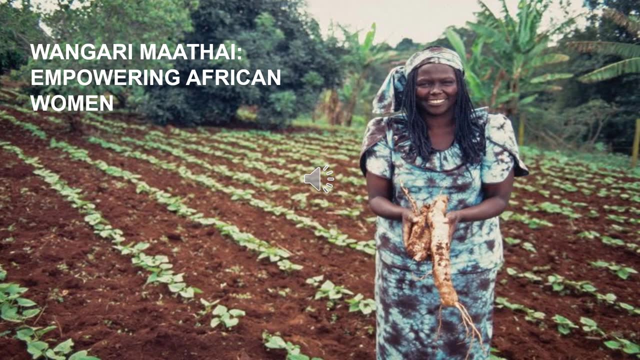 It is an endangered species native to the southeast US. It is likely on the very edge of extinction. Sightings become rarer with time. Wangari Maathai was a Kenyan environmentalist who became the first African woman to win the Nobel Peace Prize. 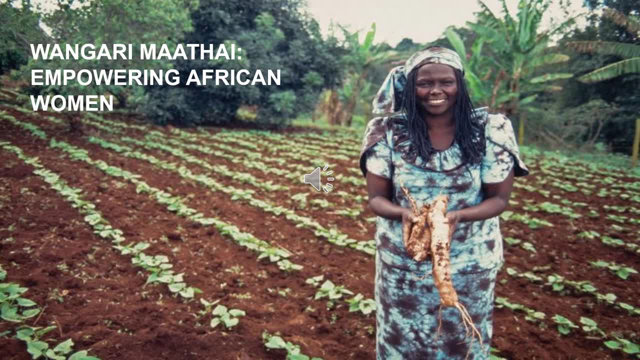 She founded the Green Belt Movement and had trees planted to combat erosion, create firewood and provide jobs for women. She mingled with people in the slums, heads of state and provided help to over 900,000 women. Exposure to lead-tainted water can cause long-term health impacts. 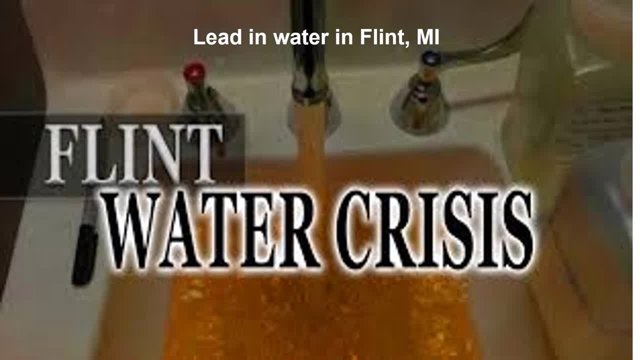 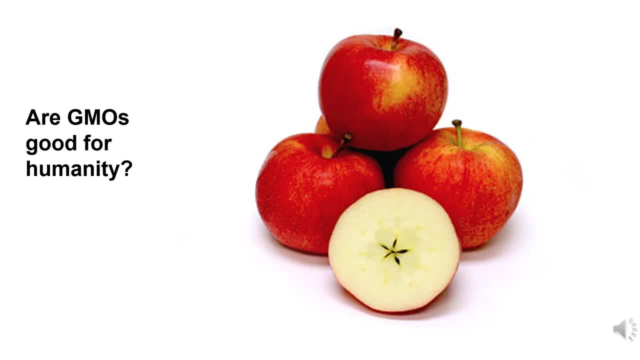 It is an irreversible neurotoxin. It creates psychological and physical damages. Genetically modified crops can be beneficial due to their resistance to insects, high crop yields, as well as a tolerance to herbicides and environmental changes. A report by PBS stated that GMOs pose more of a problem to agriculture than they do to 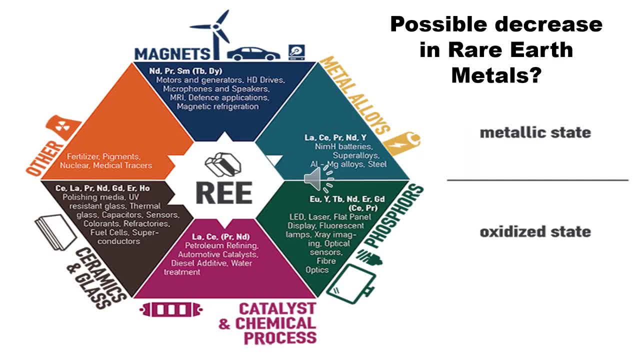 agriculture if maintenance practices are not followed. Rare earth metals are non-renewable resources that consist of the 15 lanthanides and scandium in yttrium. The metals are actually quite plentiful. however, they are dispersed and not found in economically. 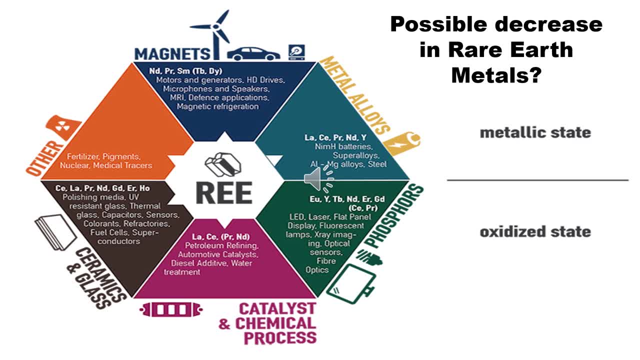 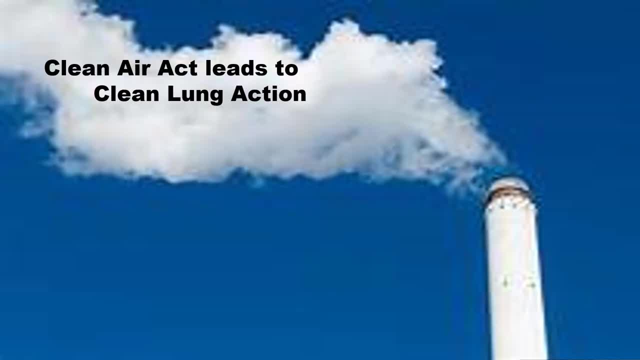 exploitable deposits. These metals are quite common in electronics, so as the quantity decreases, we will have to find more materials to replace them. In the 1960s, the public waged war on toxic metals. The government has been chinning these materials since the 1960s. 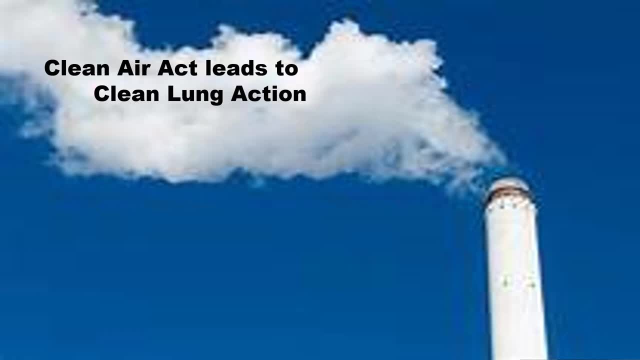 Some of the minerals are not clean. Some have some peculiarities: chemicals. in America, A lack of regulation on air quality had created toxic environments around factories that had obvious effects on human health and the environment. The Clean Air Act of 1970 is 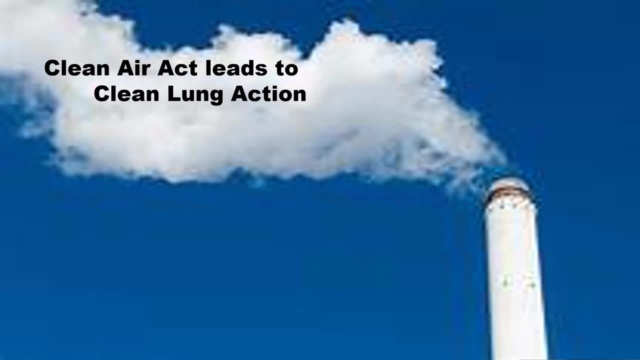 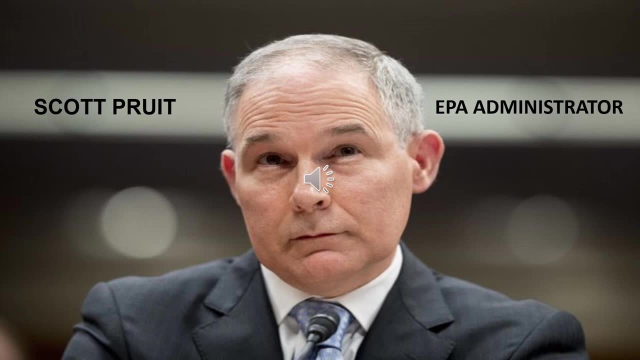 arguably the most influential piece of legislation regarding air quality ever. After being selected to run the EPA by Donald Trump, Scott Pruitt steered the agency away from environmental concerns towards business interests, with a focus on deregulation. In direct contradiction to his own administration stance, he has stated that he does not agree that carbon dioxide is a primary 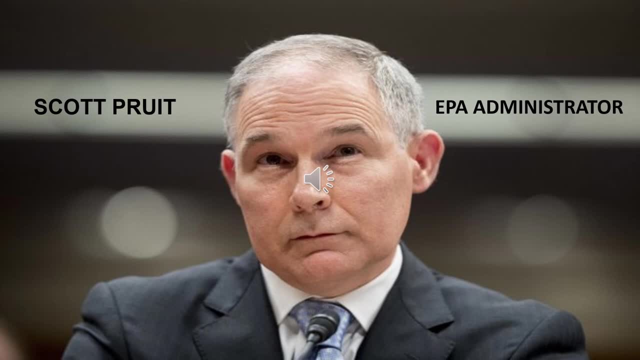 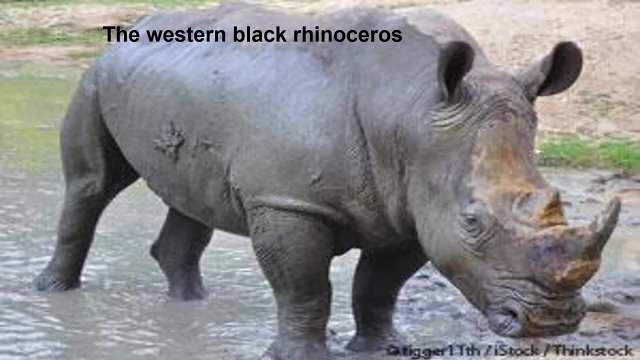 contributor to global warming. Even though he faces numerous accusations of corruption and abuses his office, he remains in his position as championed by a president who has called global warming a Chinese hoax. The Western Black Rhinoceros roam southeast region of the continent of Africa. 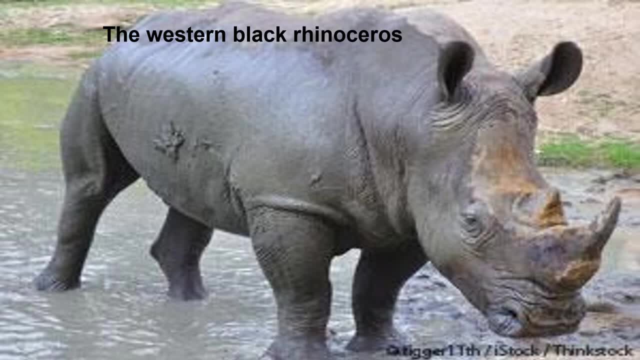 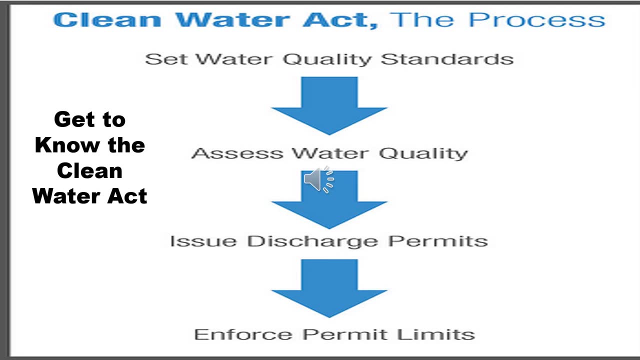 They were declared extinct in 2011 due to over poaching. The Clean Water Act first proposed in 1948, with amendments to the Clean Water Act, Amendments finally coming about in 1972.. It is the government's primary federal law governing water and pollution. The act created a building block for the regulation of pollutant discharge into the waters and regulating quality standards for surface waters. 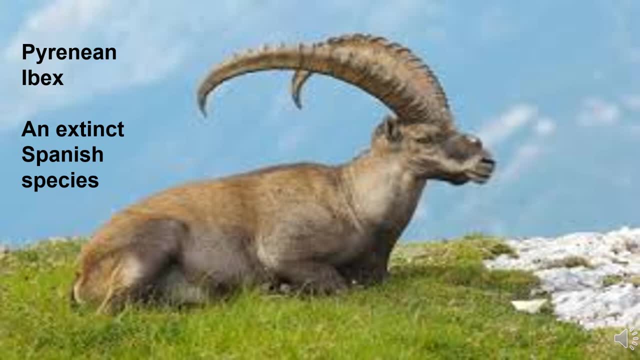 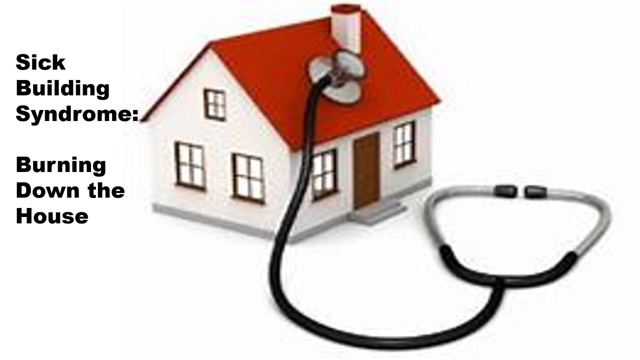 Pyrenean ibex is a now extinct subspecies of ibex that roam the Iberian Peninsula. They were common in the Canterbury Mountains, southern France and northern Pyrenees. This species went extinct January of 2000.. Sick building syndrome is when a group of people are exposed to pollutants in a common building. It is very common for buildings to be contaminated. 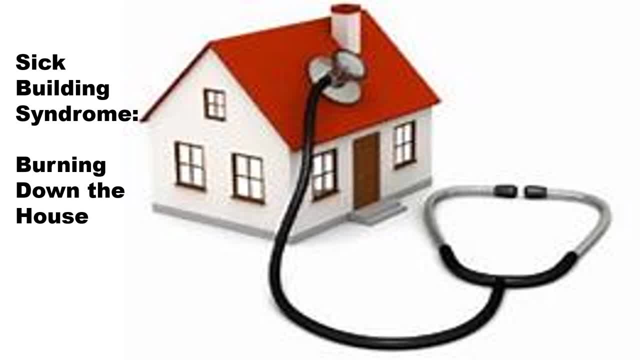 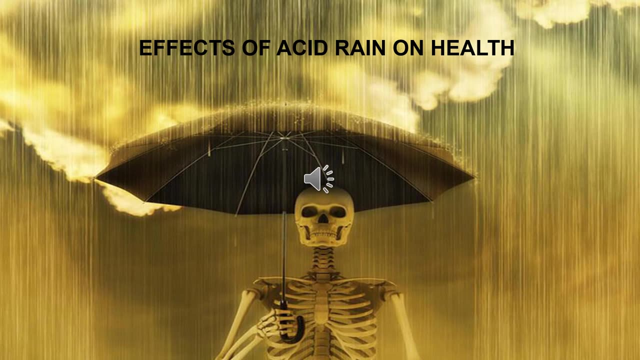 These pollutants are constructed from toxic materials, and these materials unfortunately become particulates in the air and end up being breathed in. Poor ventilation only escalates the problem. Normal rain has a slightly acidic pH of around 5.6, because of the presence of carbon dioxide. Burning fossil fuels can result in more acidic rain, though, because byproducts of sulfur dioxide and nitrogen oxides are released into the atmosphere, where they react with water and oxygen to form acids that fall to the ground or into the air. 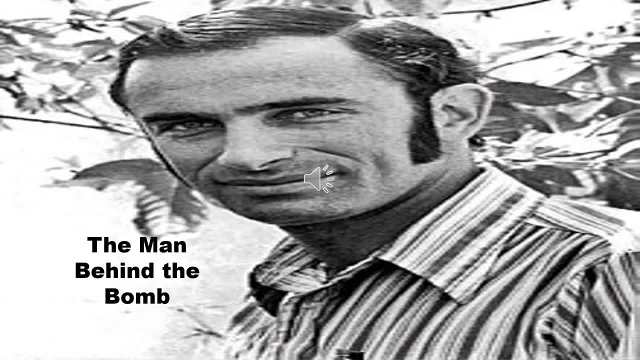 These pollutants are then transported into the atmosphere through lakes and streams or in lakes and streams, contaminating entire ecosystems. Paul Ralph Ehrlich is an American biologist and professor at Stanford University. Ehrlich's main focus of attention was in the idea of overpopulation and limited resources. 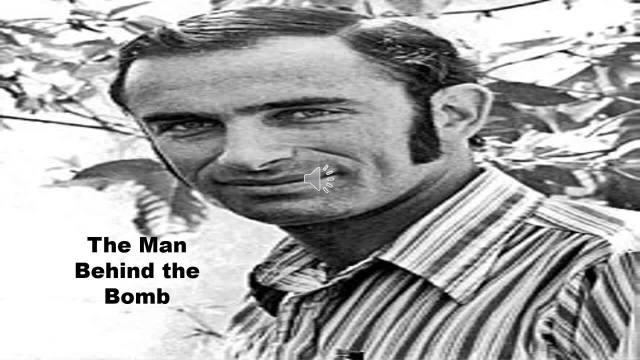 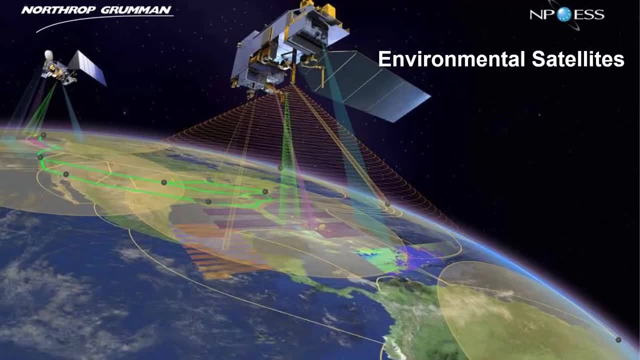 His book The Population Bomb, written in 1968, theorized that the human population would increase to the point of mass starvation. Environmental satellites are used to help monitor atmospheric phenomena that are essential for a world like ours: weathering, forecasting, measuring greenhouse gases in the atmosphere and. 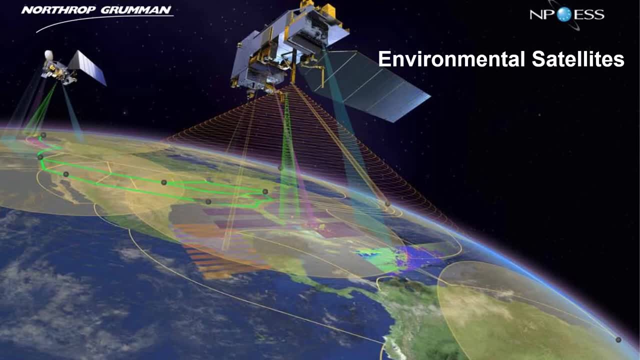 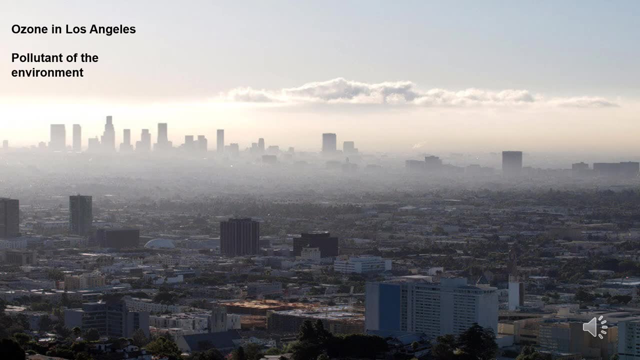 can capture high-resolution images across the atmosphere, lands and ocean, leading to better predictions. Los Angeles has reached a new high in environmental pollution due to the elevated levels of ozone located in the area. Ozone is a highly reactive molecule and can damage the respiratory tract when breathing, as well as crops and 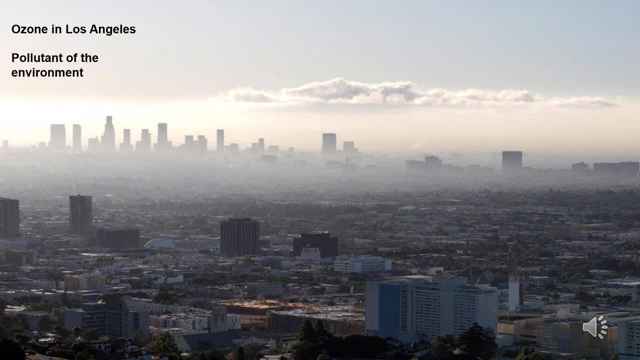 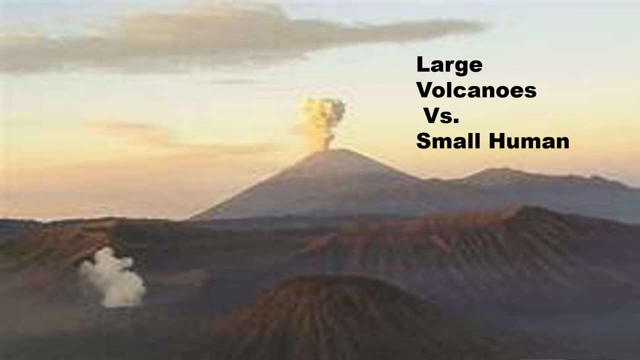 other forms of vegetation. Carbon dioxide is a well-known greenhouse gas. It is far less harmful than methane, but nonetheless harmful. The US Geological Survey estimates that human activities release over a hundred and thirty times the carbon dioxide emitted by volcanoes, both sub-aerial and submarine. The frack.